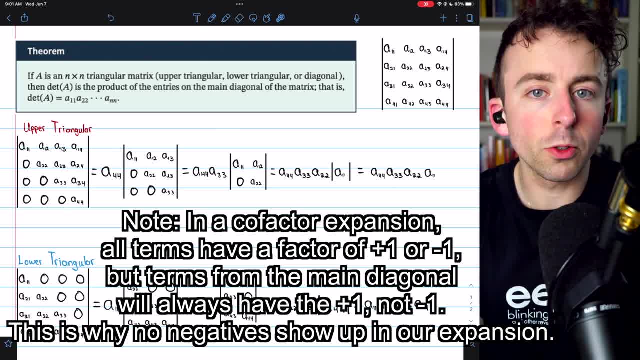 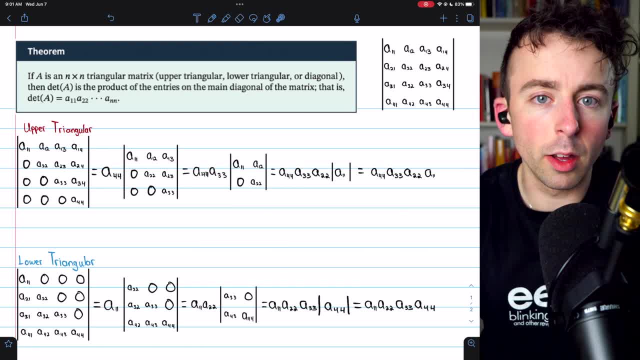 see why it's true. Here is a general example of an upper triangular matrix. What is the determinant of this matrix? Well, we could calculate it using the cofactor expansion of any row or column. This bottom row has all zeros, except for the last entry. 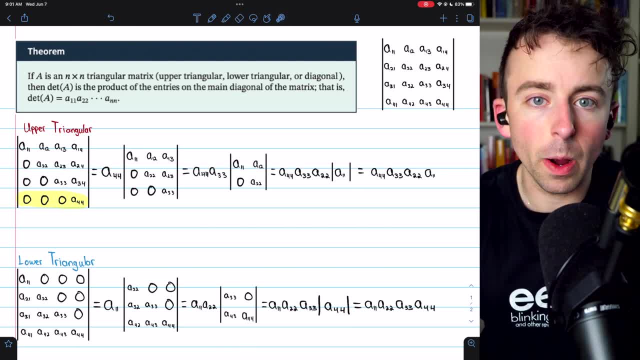 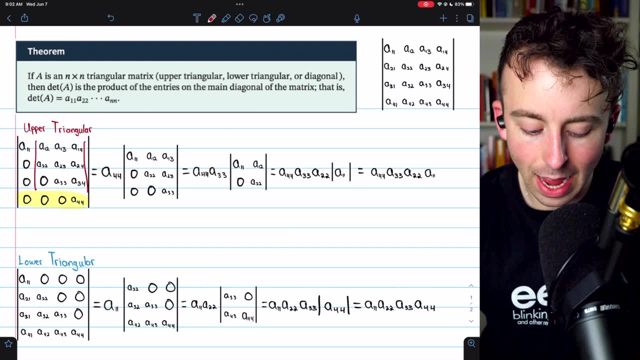 so that'll be easy. Let's do the cofactor expansion of that row. Then the determinant will be this first entry, zero times the determinant of this minor matrix, and that's just going to be zero. It will be similar for this entry: zero. Similar for this. 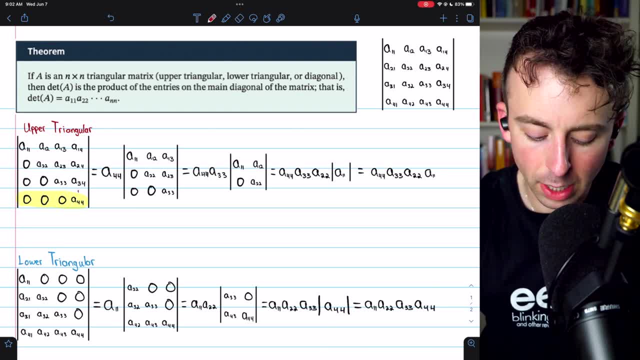 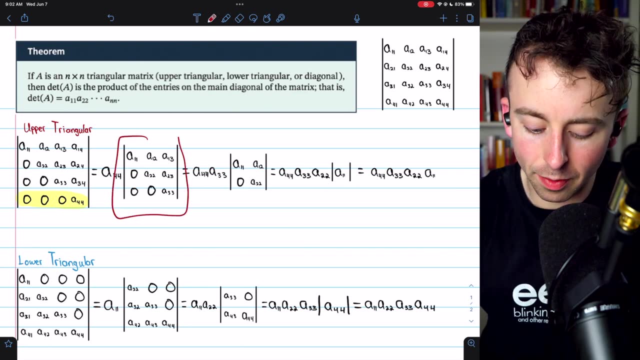 entry zero And then, finally, the only non-zero term will be this entry multiplied by the determinant of this sub-matrix, And that's what you see here. So we have a44 times the determinant of that sub-matrix. So then, what is the determinant of this sub-matrix? Well, we can. 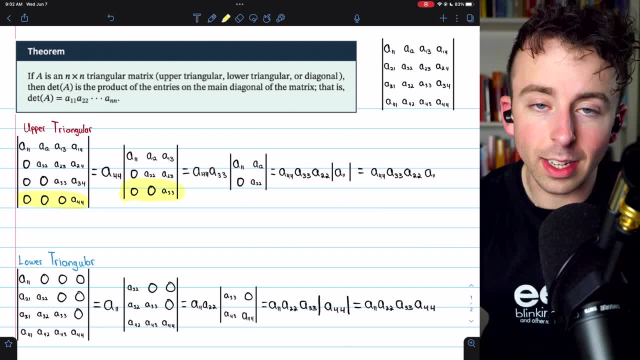 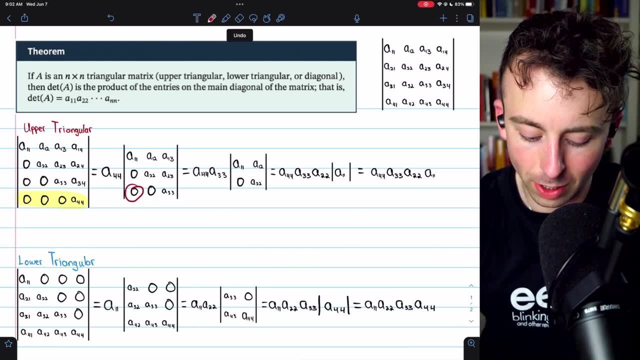 calculate that with a cofactor expansion- And this third row is easy to use because it's mostly zeros. Again, we would have zero times a determinant of that sub-matrix. Same thing here. it'd give us another zero And then we would multiply by a33 and multiply that by the. 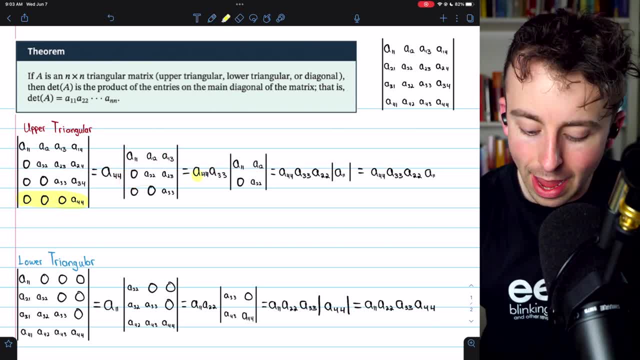 determinant of this sub-matrix. Now we have a44 times a33, both parts of the main diagonal, and that's getting multiplied by the determinant of this matrix. We can continue the cofactor expansion. We'll use this row since it has zero. The zero is just. 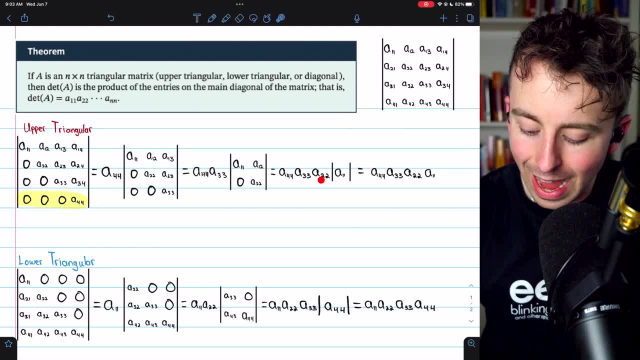 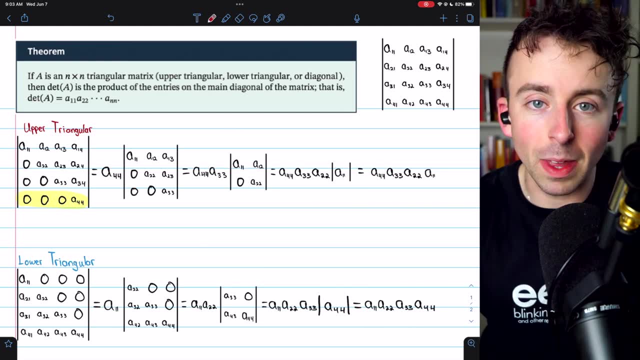 going to give us a zero. And then we need to multiply by a22 times the determinant of this sub-matrix. That's just the determinant of a single entry and the determinant of that, by definition, is just that entry. So by applying the cofactor expansion definition of the 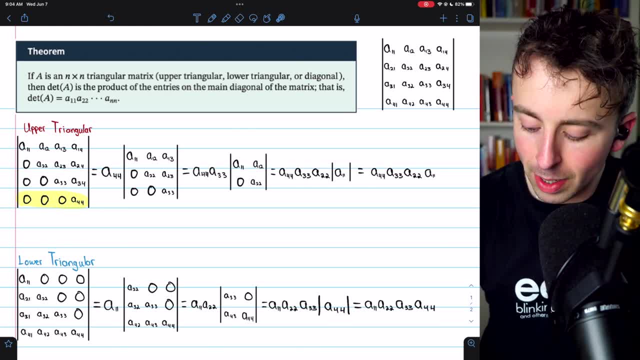 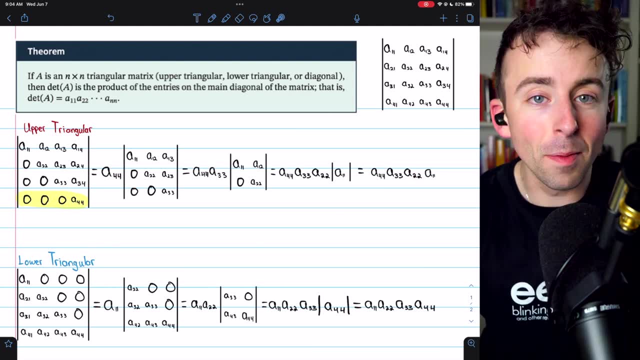 determinant to this matrix. we find that its determinant is a44 times a33.. That's a33 times a22 times a11.. It's just the product of the entries on the main diagonal. Pretty nice. And here is more or less the same exact process written out for: 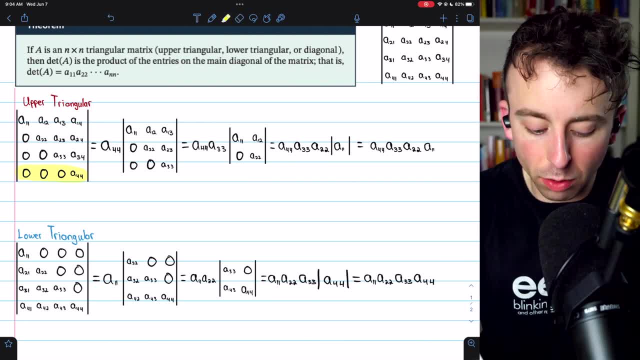 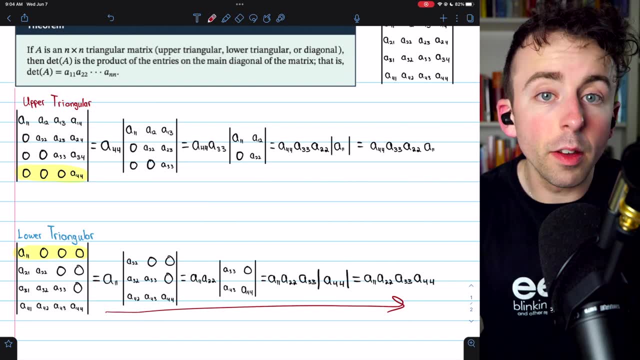 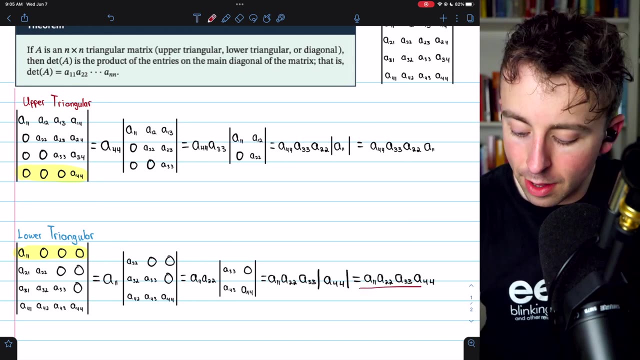 a lower triangular matrix. In this case, we use a cofactor expansion of the top row, because that's the one with the most zeros, and this proceeds in very much the same way. As you can see, the only entries that actually come into the computation here end up being the. 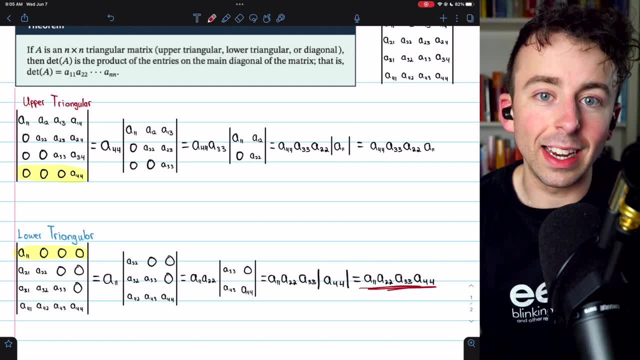 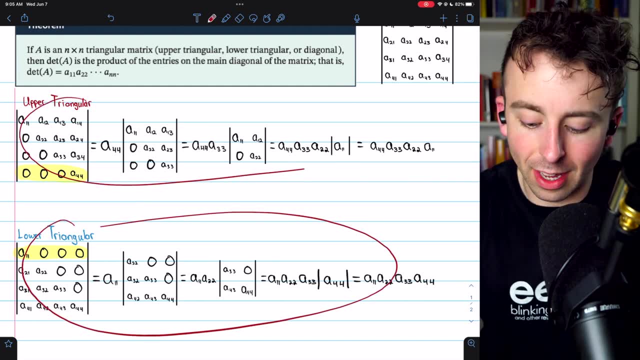 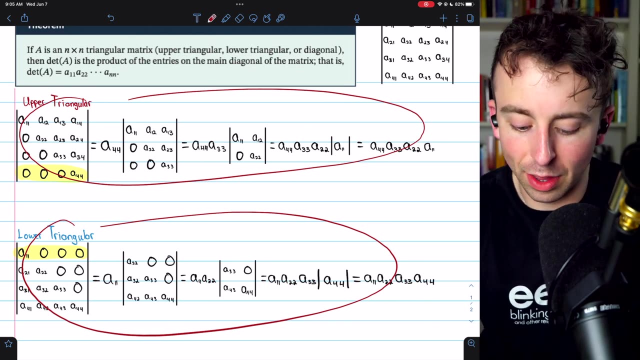 entries that are on the main diagonal. So if we consider just a diagonal matrix that has zeros outside of the diagonal, well, the computation is still going to be the same as these, because the only entries that affect the computation are those on the diagonal. So if we turn everything, 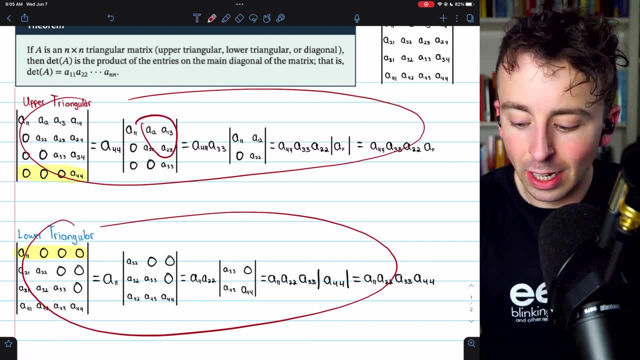 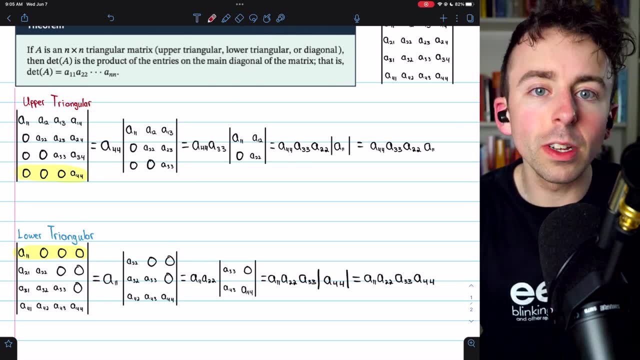 else to zeros, to make it just a diagonal matrix. well, we're still going to get the same thing. So for a diagonal matrix this still applies. Its determinant is just the product of the entries on the main diagonal. Let's do some examples. These exercises are from Howard Anton's Linear Algebra Text. 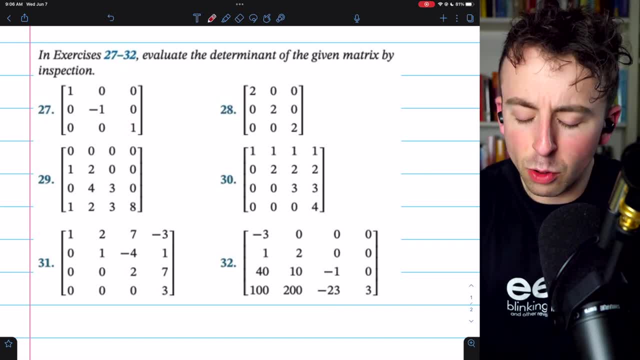 Link in the description if you're interested in that. We're just asked to evaluate the determinant of the given matrix by inspection, which means it's really easy. You can pretty much just look and calculate it in your head, because these are triangular matrices, So we can apply the theorem. 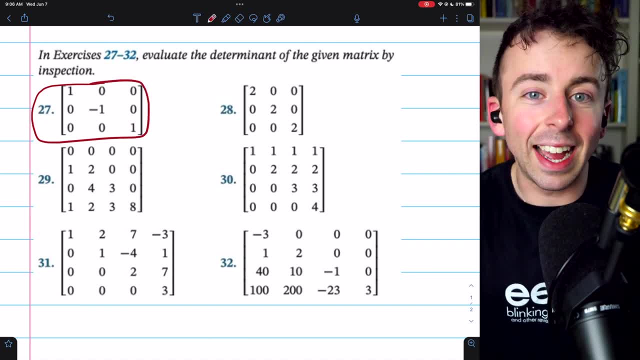 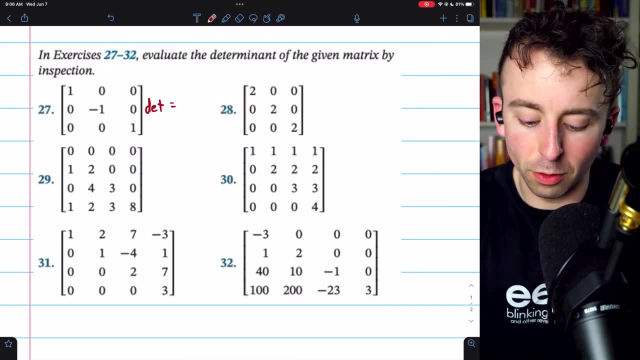 that we just learned. Here is problem 27.. It's a diagonal matrix. Its determinant is just the product of the entries along its diagonal. We'll use some sloppy notation here and just write for determinant. I won't bother with names. We don't have a ton of space here, So just multiply. 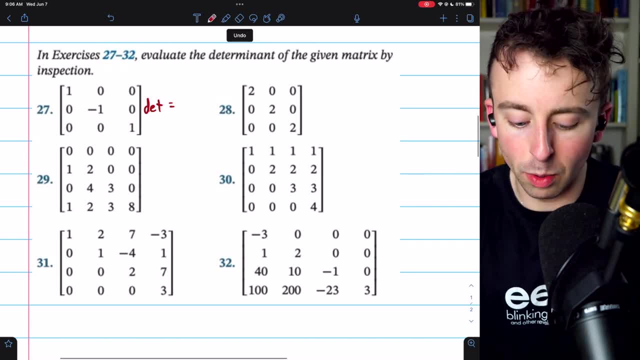 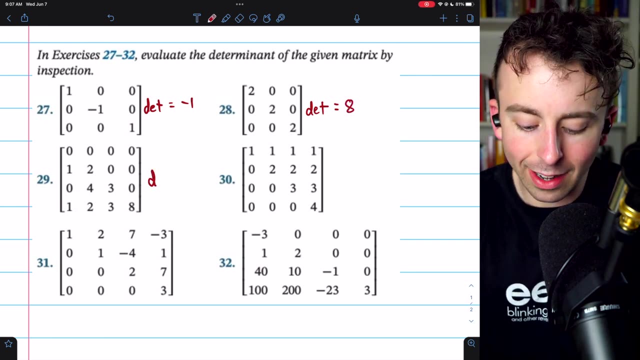 all these entries 1 times negative. 1 is negative 1. And when we multiply that by 1, we get negative 1.. That's the determinant. The matrix in problem 28 is also a diagonal matrix. Its determinant can be found by just multiplying across the main diagonal. That's 2 cubed, which is 8. 29, we have. 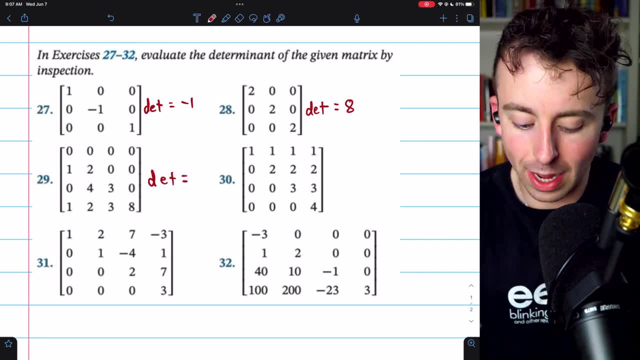 a lower triangular matrix, Its determinant can be found by just multiplying across the main diagonal. See that's going to be 0.. Any time that a matrix has a row or column of all zeros, its determinant will be 0, which is an immediate consequence of the cofactor expansion definition of the 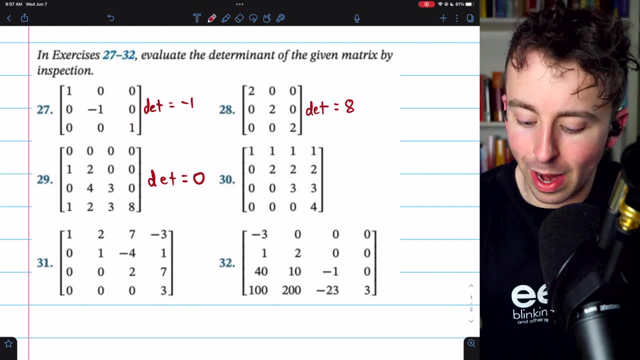 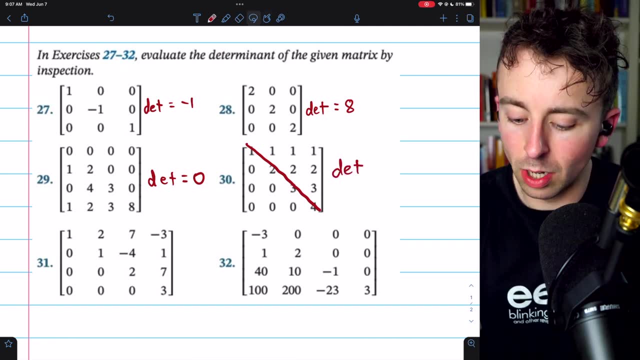 determinant. Here is problem 30. This is an upper triangular matrix. Multiply across the main diagonal in order to find the determinant. That's going to be 1 times 2 times 3 times 4, which is 24.. Problem 31. We have an upper triangular matrix. We can.